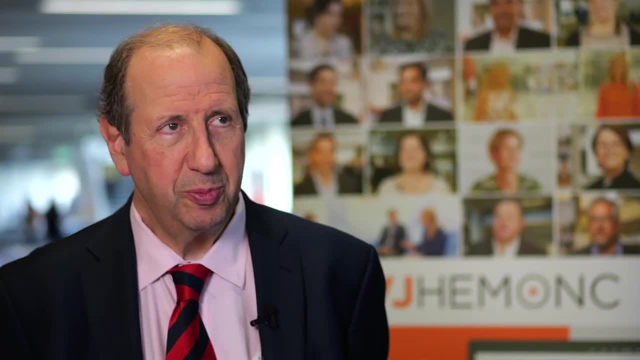 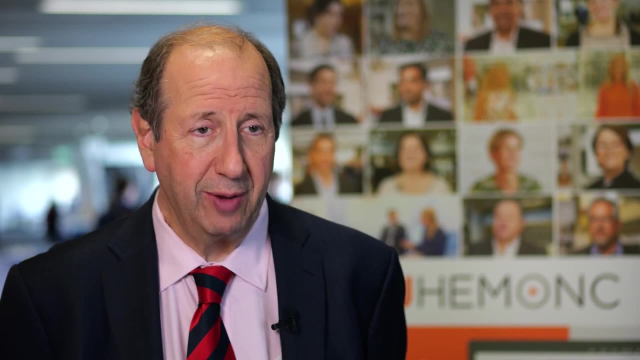 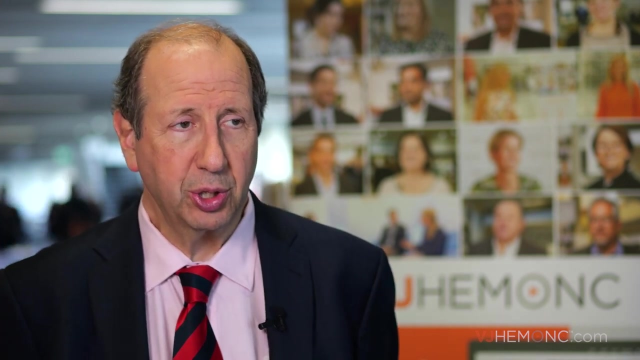 So there's been two classification systems released in 2022. One was an update of the WHO system and one was a new classification system called the ICC or International Consensus Consortium. The latter one had a few more clinicians associated with it and maybe that's. 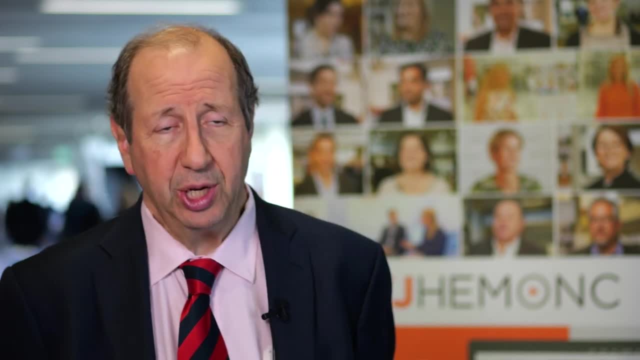 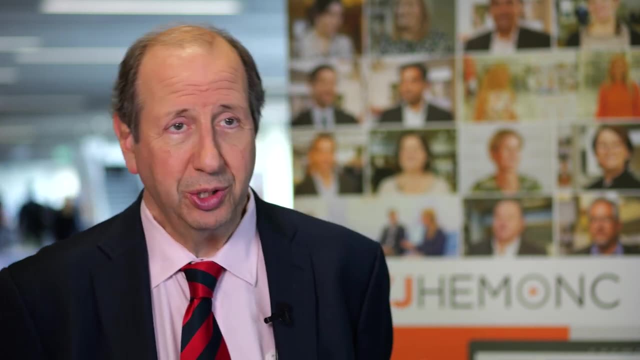 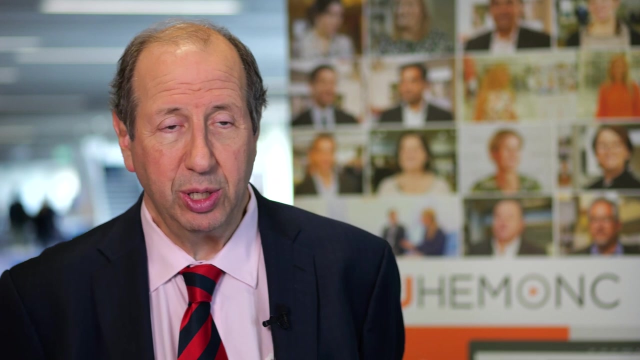 why one of the key differences between the two was that in the ICC they called out a group called MDS slash AML, which are those with 10 to 19% blasts which in the WHO, still remain in the MDS category, either IB1 or IB2, depending on the number of blasts. Also, 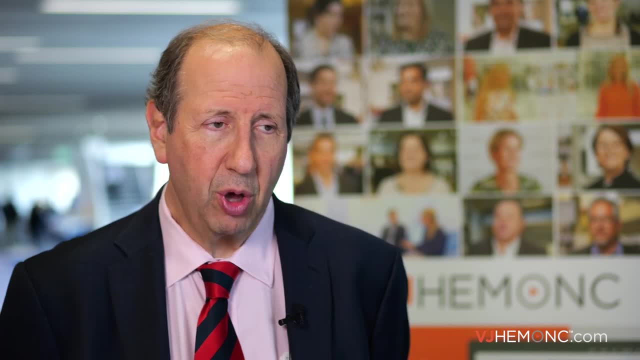 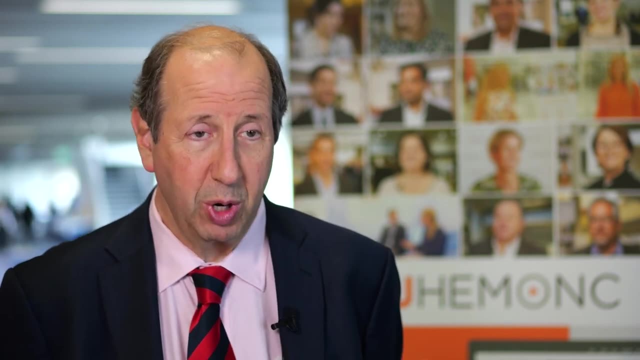 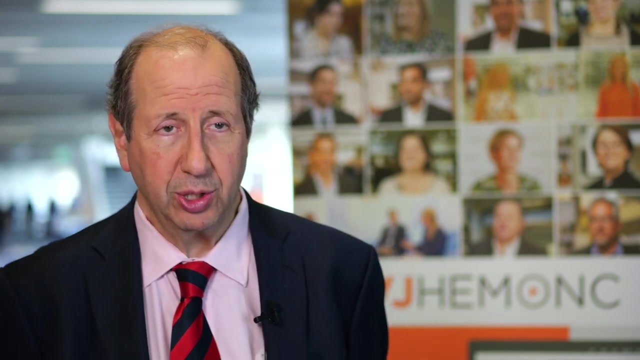 the two classifications differed suddenly in calling out patients with recurrent genetic or pseudogenetic abnormalities, because they don't require a 20% blast or even 10% blast to be called AML. as long as a patient has one of those recurrent abnormalities, such as a 6-9 or an 8-16 or even a TA-21, they can be considered. 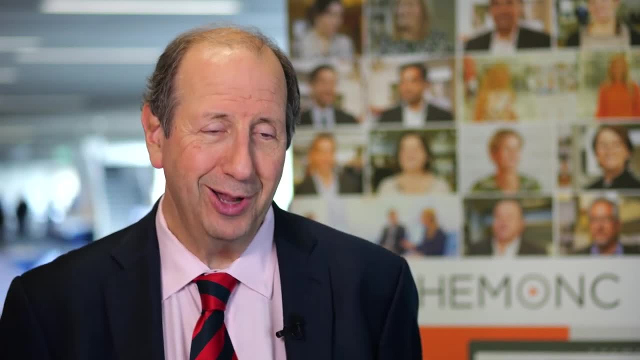 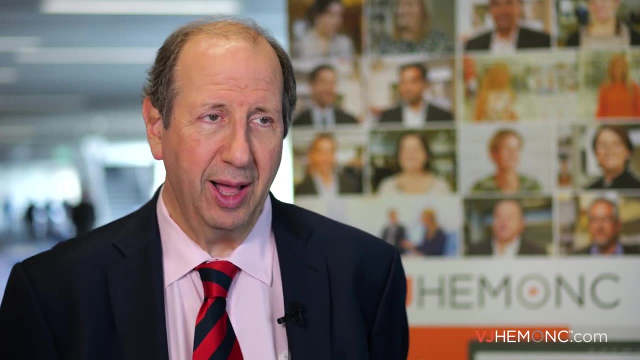 AML in the WHO if they have 5% blast or greater, in the ICC if they have 10% blast or greater. So the presence of two classification systems has caused some consternation in some circles, but I think it's really up to the clinician to synthesize all the data, no matter what. 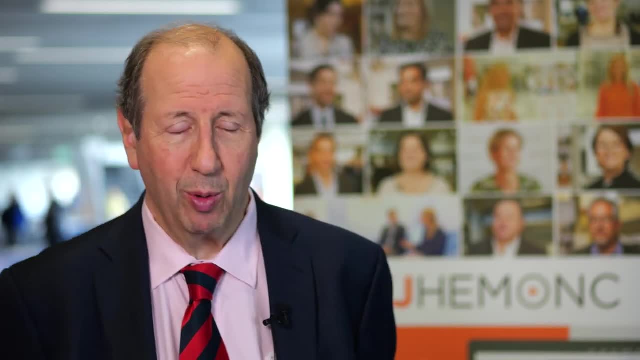 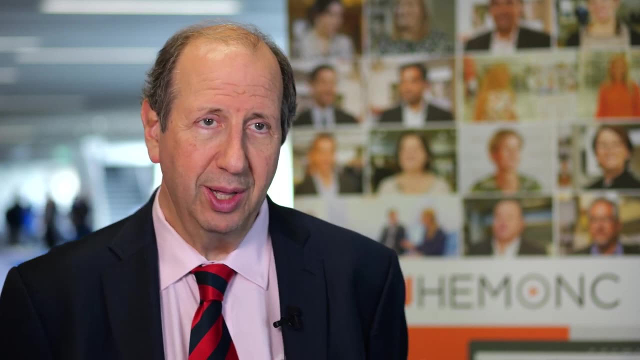 you do. I think it's really up to the clinician to synthesize all the data, no matter what you call it, which brings up the next thing and the last thing I'll talk about, which is the ELN 2022 classification system, which really is more of a prognostic issue than a pure classification issue from the pathology standpoint. 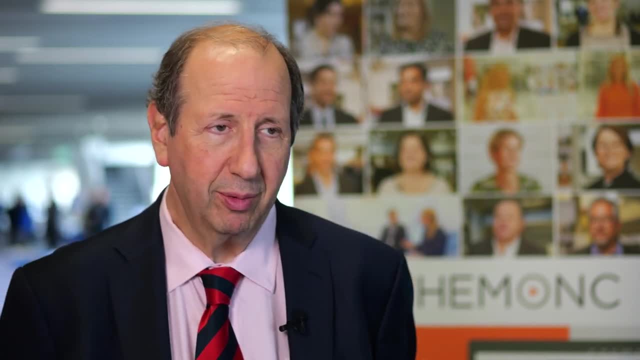 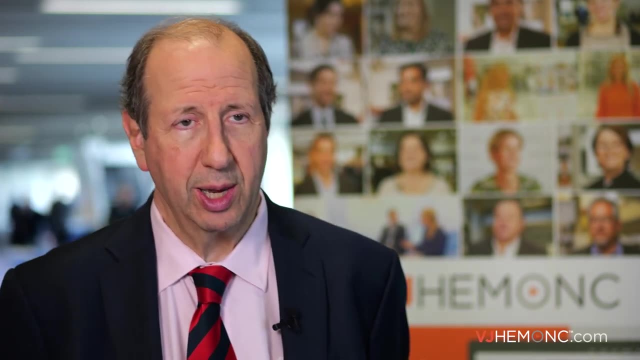 The classification. the prognostic categories do impact the way we treat patients to a certain degree, and some of the key changes in the 2022 ELN classification system have to do with FLT3 mutations, because of the advent of the FLT3 inhibitors which we talked about. 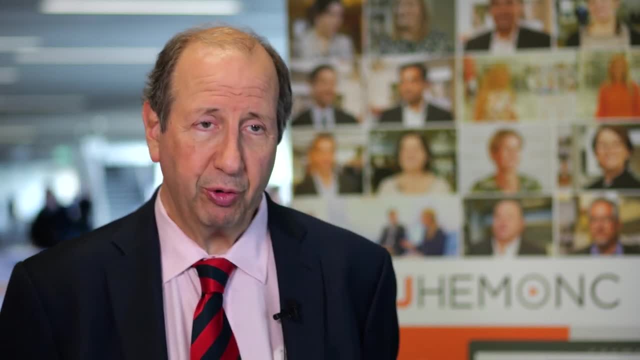 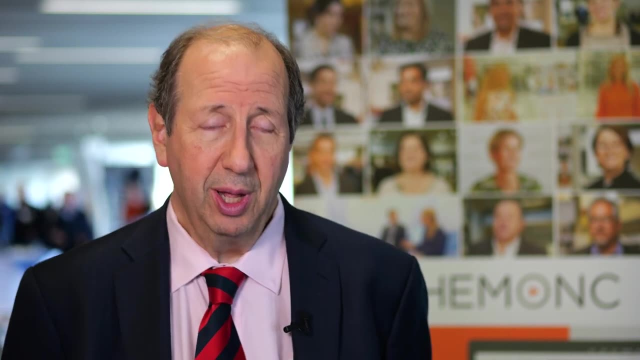 The classification, the prognostic categories, do impact the way we treat patients to a certain degree, and some of the key changes in the 2022 ELN classification system have to do with FLT3 inhibitors, which we liked to talk about Previously, those who have a FLT3 mutation, regardless of the Benson-张ke thing. Dieser aus Feibo och von Sch急, mosktyn was follows a grandpa ov.